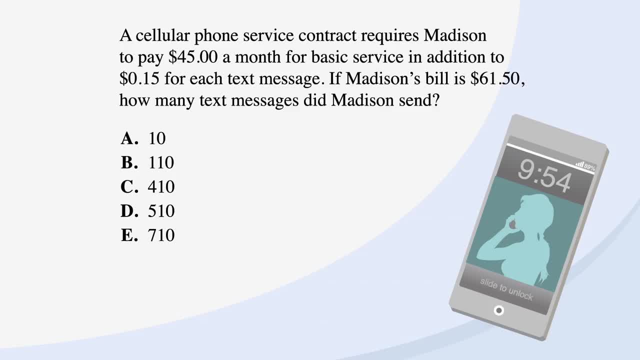 the ACT. Here we've got a question about Madison's cell phone bill, which is slightly higher than her mom would like. Madison's cell phone service contract requires her to pay $45 a month for basic service, in addition to 15 cents for each text message. If Madison's 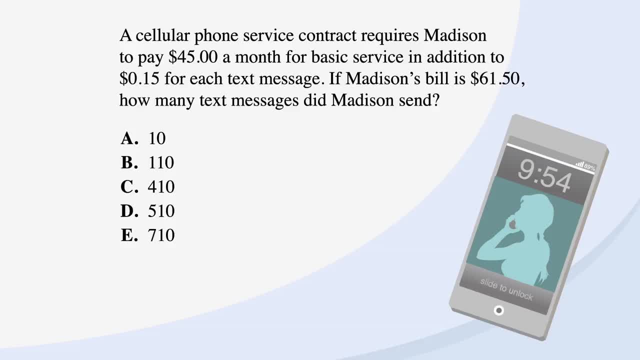 bill is $61.50,. how many text messages did Madison send? A is 10,, B is 110,, C is 410,, D is 510, and E is 710.. First we'll underline the form, Then we'll circle the keywords- How many text messages did Madison send? And label. 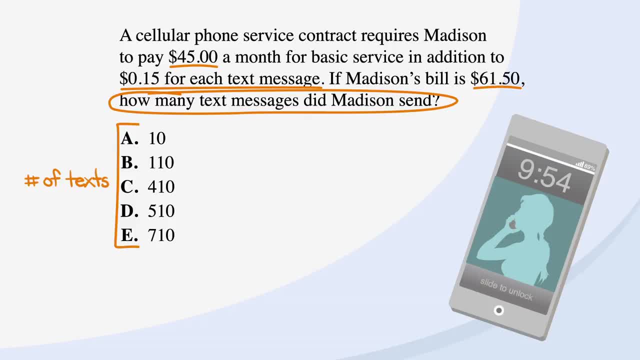 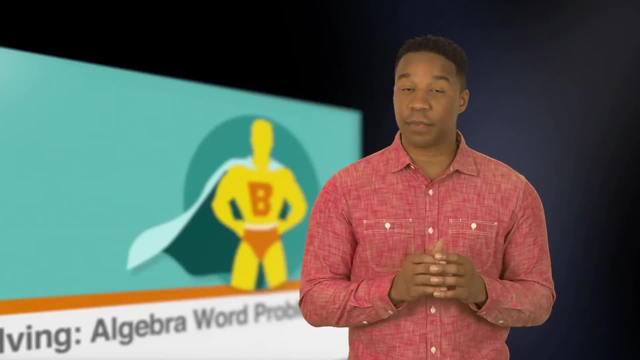 the answer choices, which represent the number of texts Madison sent This question, has verbally given us a few equations and then has asked us for the value of one of the variables in these equations. So we know we can back-solve. Now let's identify. 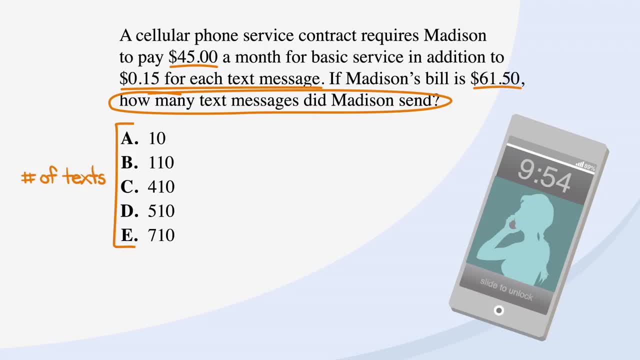 the number we're trying to get. If we plug in the right answer choice, we should get that Madison's bill was $61.50.. That's our target number. What else do we know? We're told that customers pay a base rate of $45, and an additional 15 cents per text. 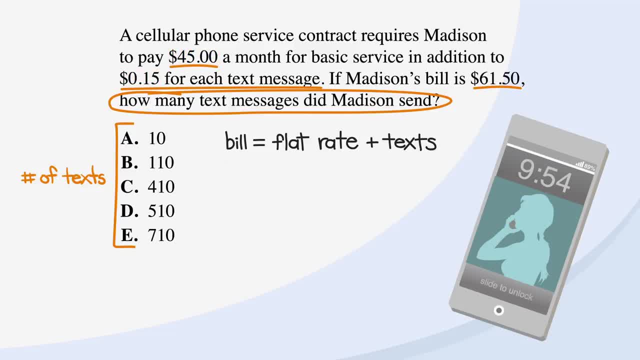 If the bill equals the flat rate plus the cost of text, we can plug in $45.00 plus 15 cents per text. We're ready to back-solve, Remember. our next step is to start with the middle choice, Answer C, and plug in the values. 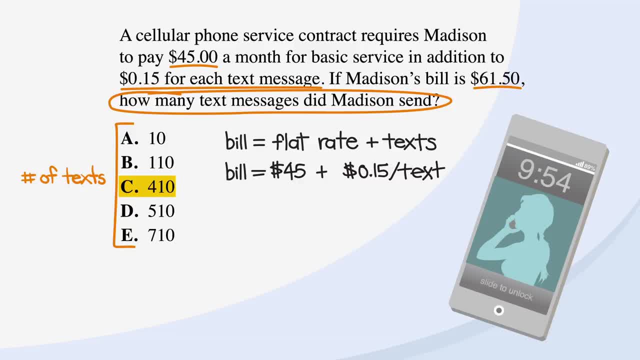 we're given in the answer choices, We'll move on tovolleycom. Okay, Give a stomp Now to wait To 55 cents. Keep it evenings. C says that our customer sends 410 texts. If Madison paid 15 cents per text, 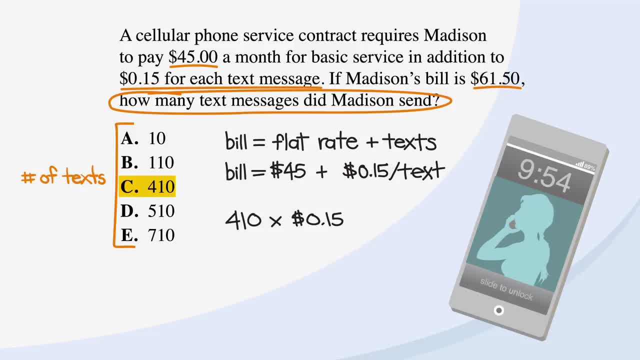 we would say that she paid 410 times 15 cents, or $61.50 for the text messages. That sounds like it matches right. Not so fast. Remember, she has to pay a flat rate of $45 per month as well.